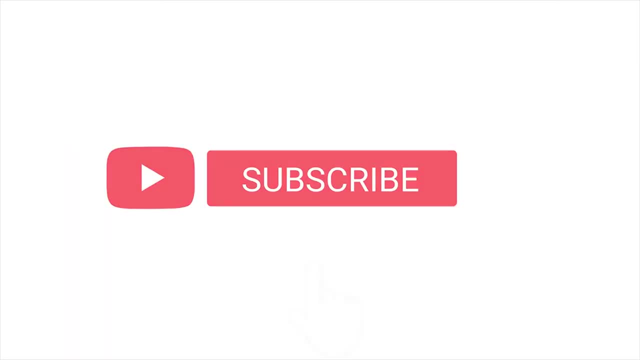 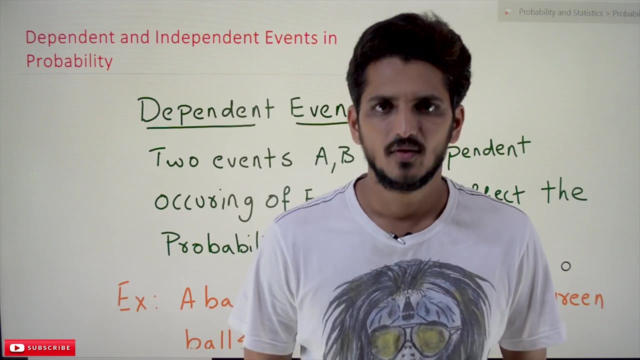 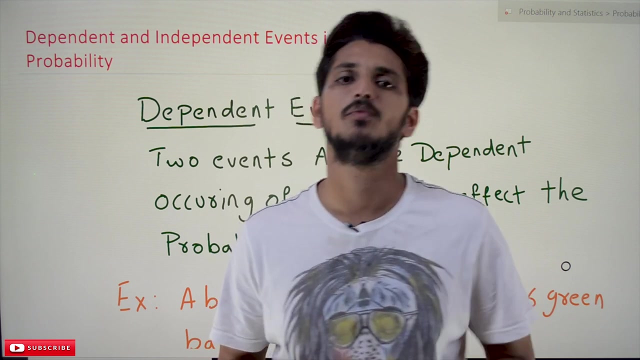 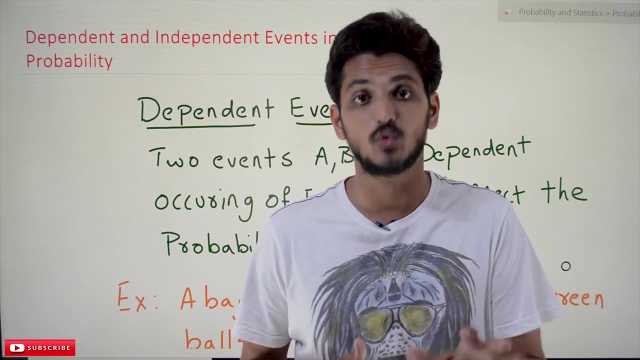 Hi, welcome to Learning Monkey. I am Raghu here. In this class we will discuss about dependent and independent events in probability. In our previous classes we have done some examples on probability using combinations, probability using union. Please watch those classes, They will help you. 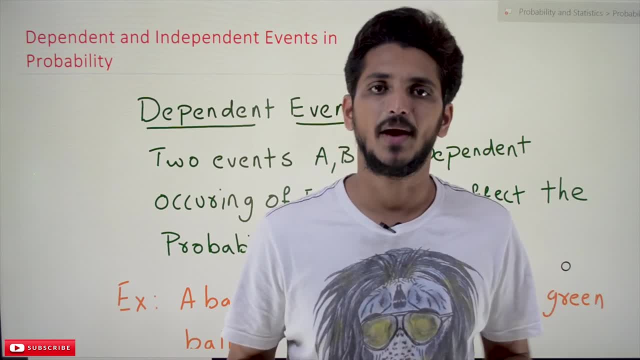 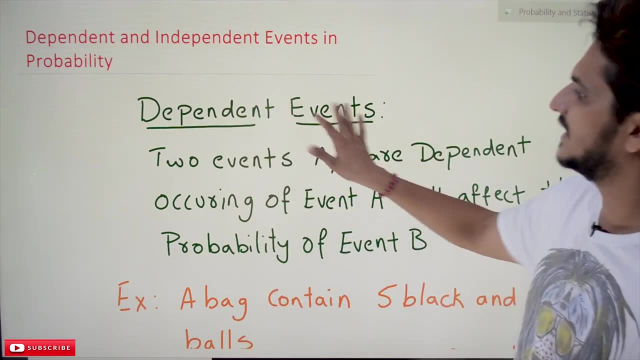 a lot in understanding this class. Please watch those classes and come back here. The link for the playlist is provided in the description below. Coming to today's class, first, we are going to understand dependent events. We will take an example and understand for better understanding. 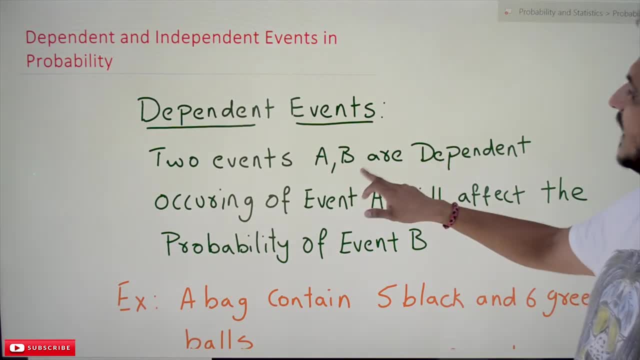 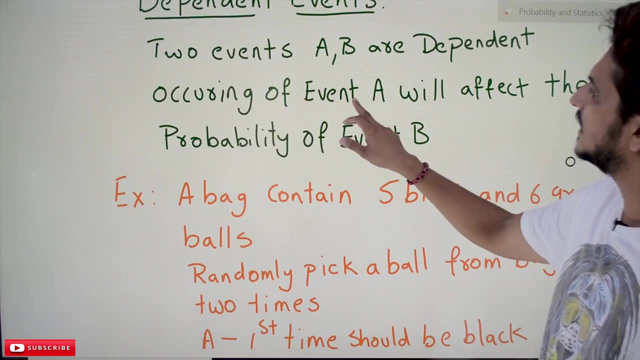 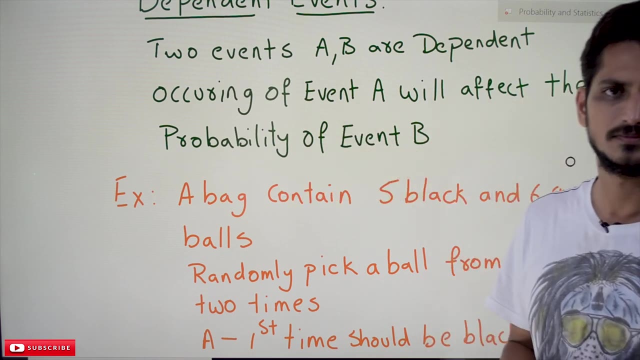 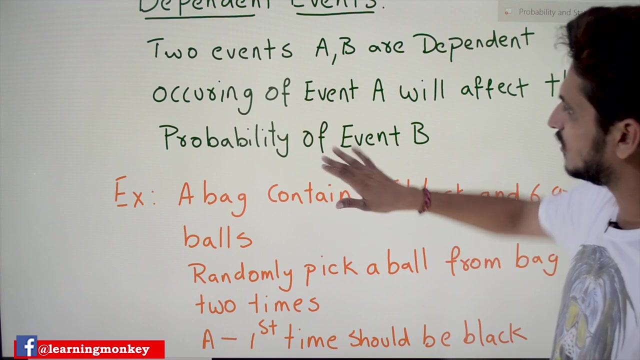 With example we will have a better understanding. Two events, a comma b, are dependent events. When we are going to say there are two events are dependent events occurring of one event, event a will affect the probability of event b. Then we can say that the two events are dependent events. Now, with example you will get: 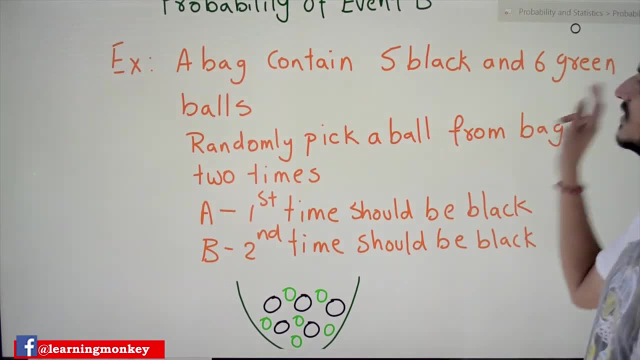 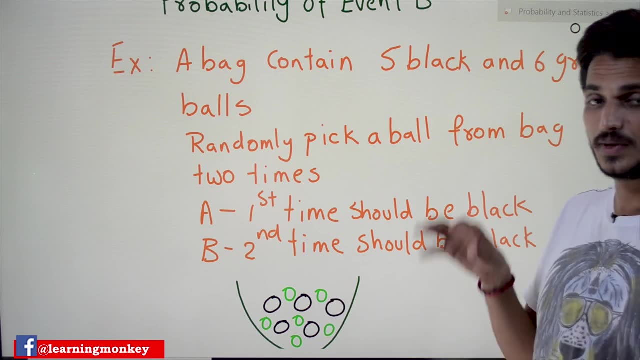 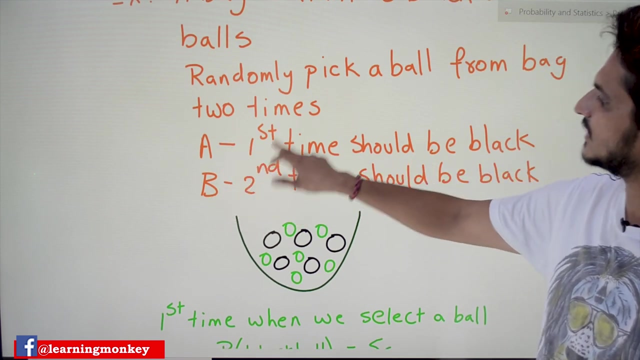 clarity. A bag contains five black balls and six green balls. Randomly pick a ball from the bag two times. So we have to pick a ball from the bag two times. That is what we have to do. So what is the events? Events a- b are saying that a first time should be a black ball. 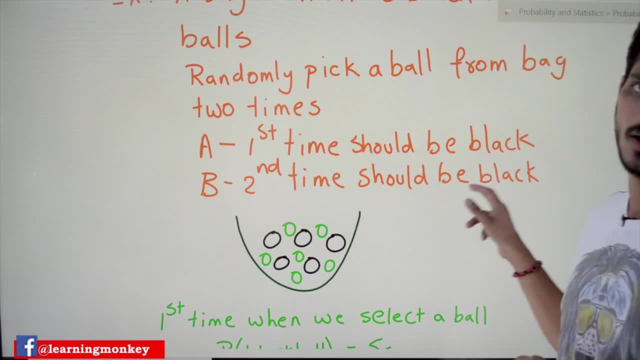 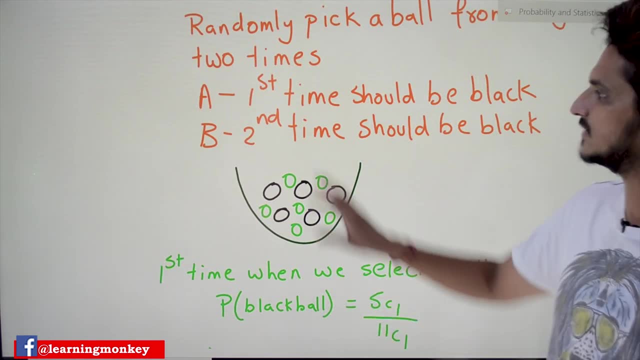 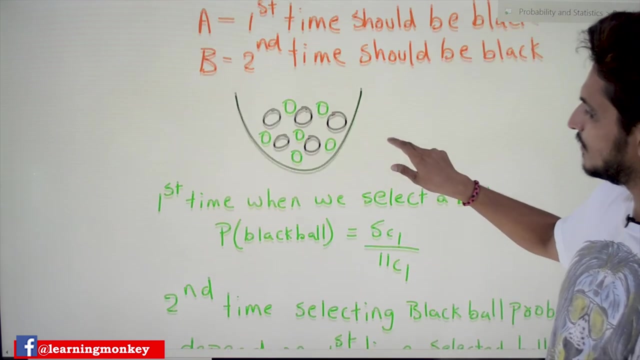 Event b says that a second time should be a black ball. So what happens if you want to do this action, if you want to do this experiment? what happens? First time it should be a black ball. How many balls are there Total? five plus six. Eleven balls are there? Total combinations are: 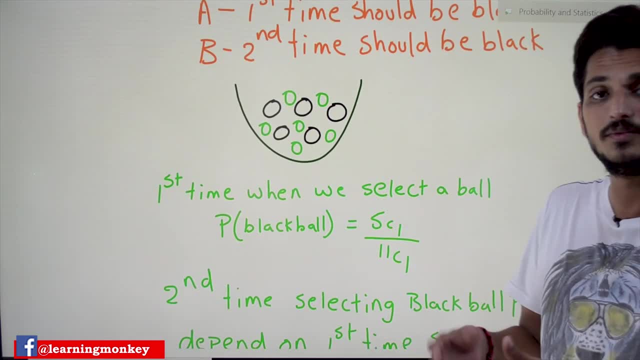 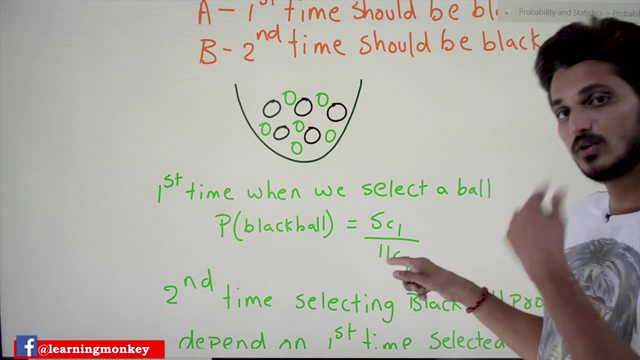 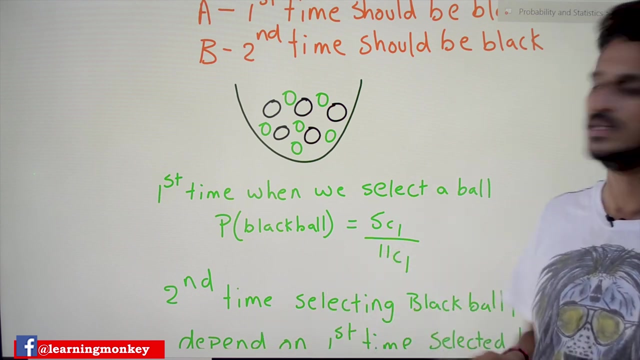 eleven c one means our sample space is eleven c one, We can pick a ball. The ball is having eleven c one. possibilities means our sample space. These discussions were made in our previous class. Out of that, how many black balls are there? Five black balls are there, So five c one by eleven c one. 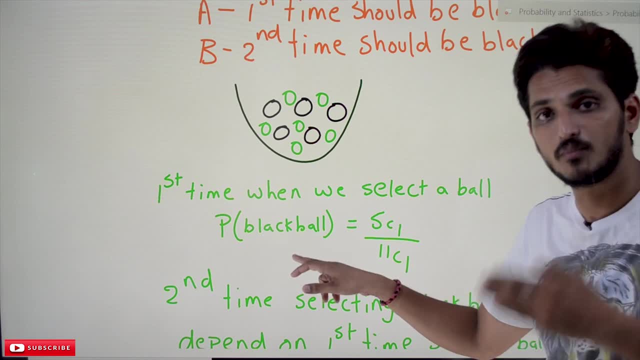 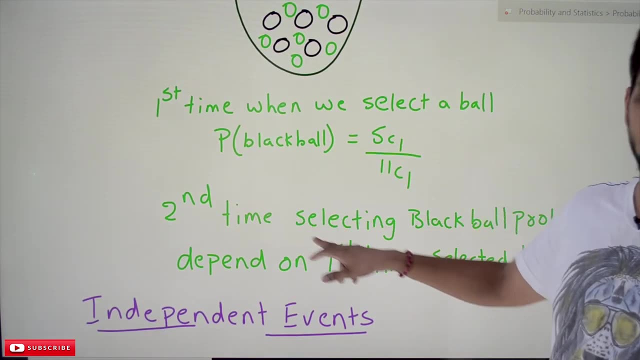 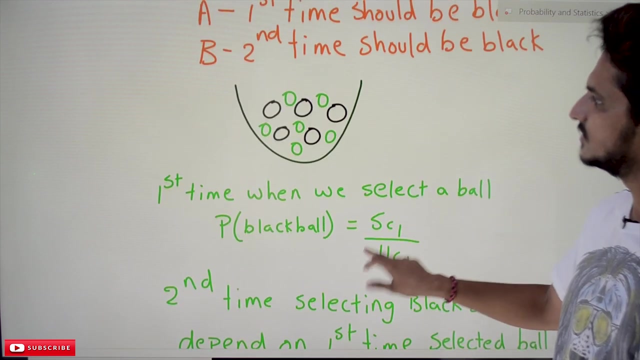 is our probability that we are going to pick a black ball in first time. But if you, if you consider the second time selecting black ball, probability depends on first time selection. Means see first time. if you pick the green ball, the probability that a second time you will pick a black ball is. 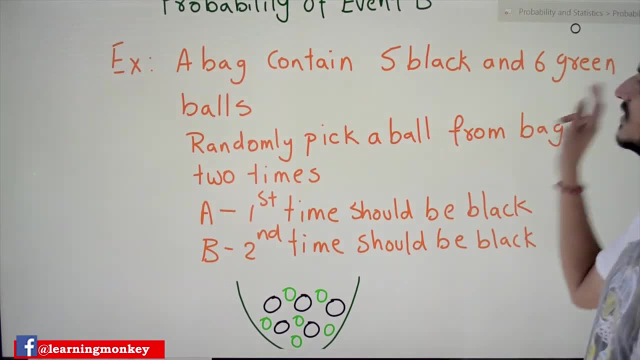 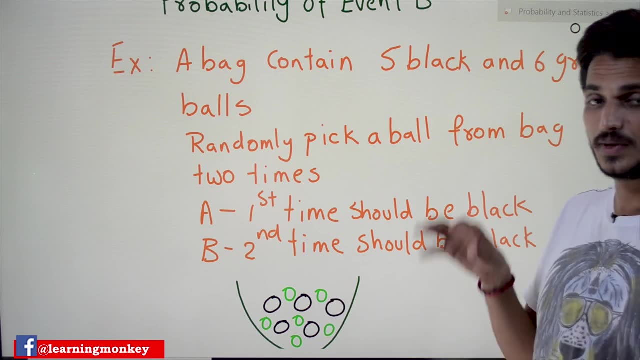 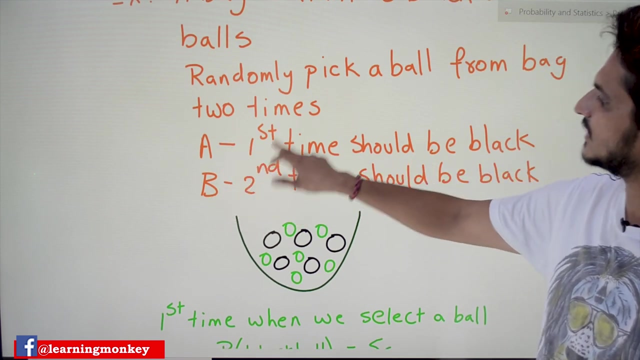 clarity. A bag contains five black balls and six green balls. Randomly pick a ball from the bag two times. So we have to pick a ball from the bag two times. That is what we have to do. So what's the events? Events a- b are saying that a first time should be a black ball. 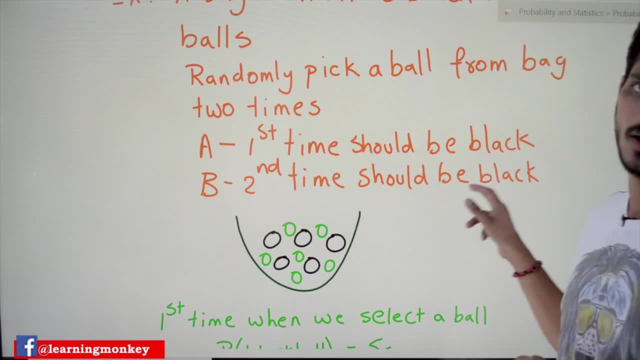 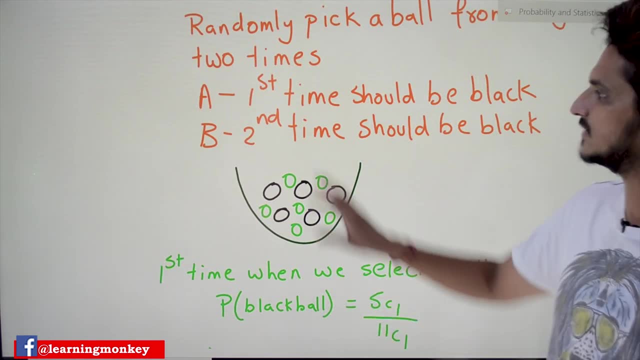 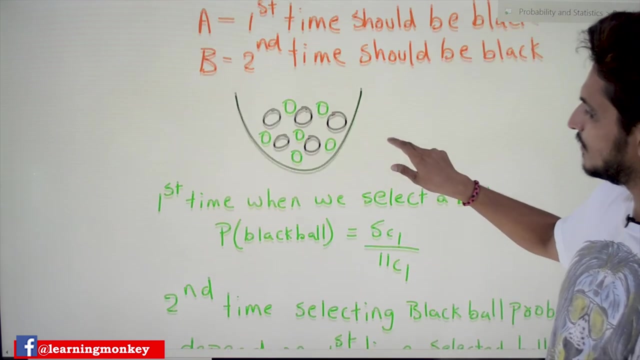 event b says that a second time should be a black ball. So what happens if you want to do this action, if you want to do this experiment? what happens? First time it should be a black ball. How many balls are there Total? five plus six. Eleven balls are there? Total combinations are: 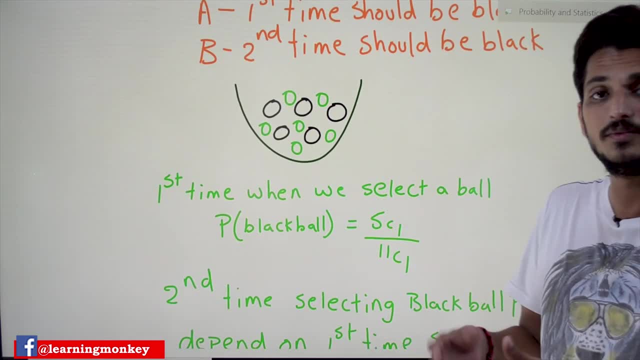 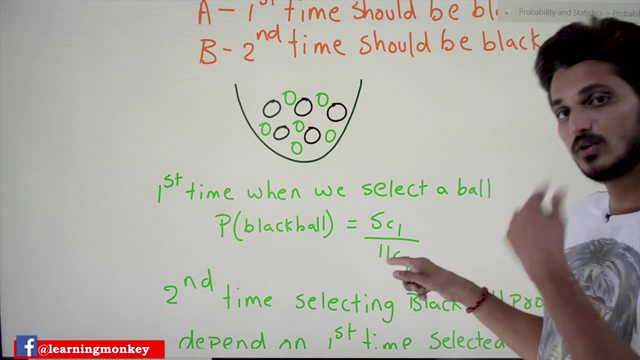 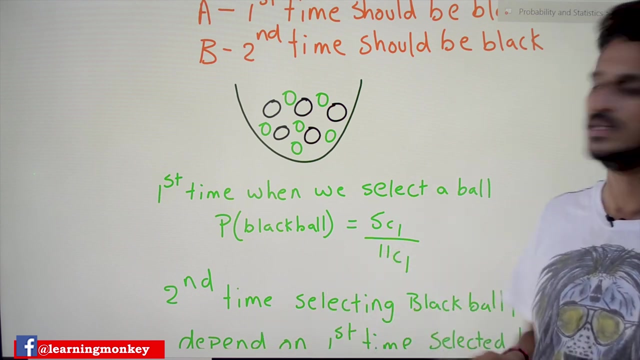 eleven c one means our sample space is eleven c one, We can pick a ball. The ball is having eleven c one. possibilities means our sample space. These discussions were made in our previous class. Out of that, how many black balls are there? Five black balls are there, So five c one by eleven c one. 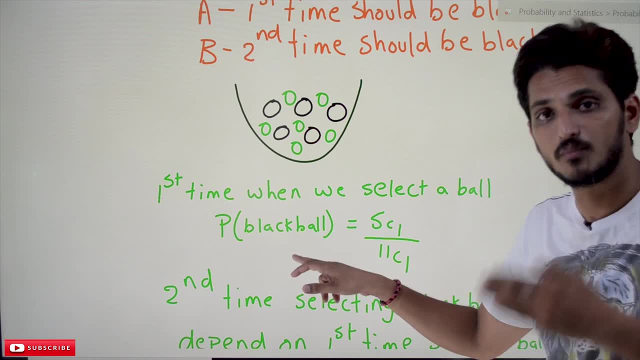 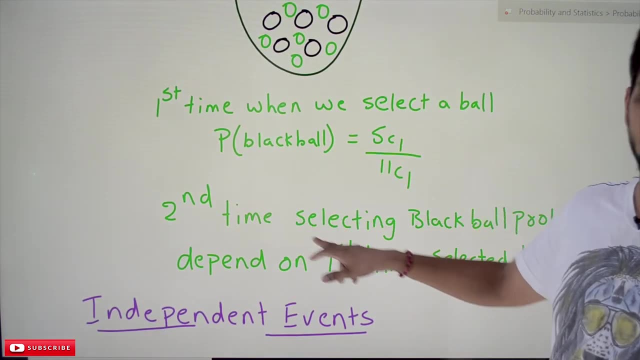 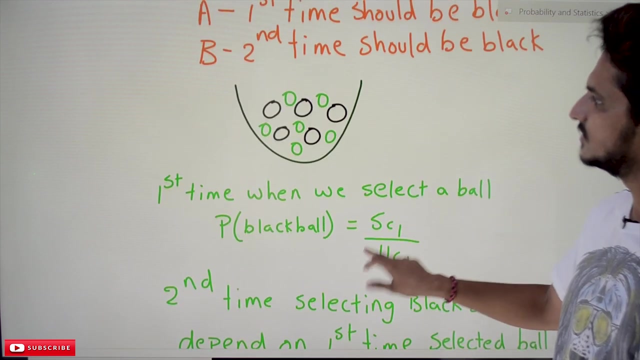 is our probability that we are going to pick a black ball in first time. But if you, if you consider the second time selecting black ball, probability depends on first time selection. Means see first time. if you pick the green ball, the probability that a second 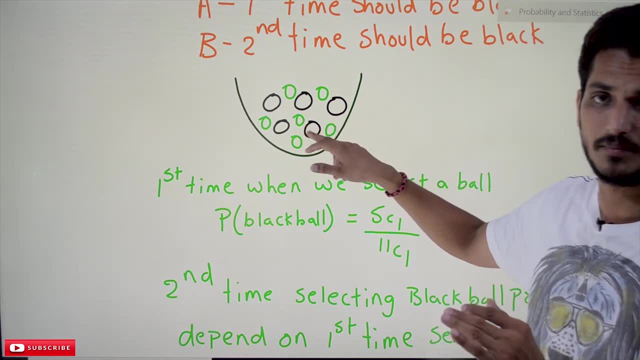 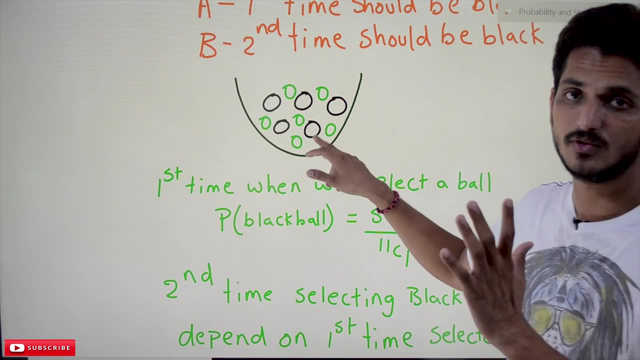 second time it is going to. you are going to pick a black ball is different, Because if you pick a green ball from this, how many balls remain? Total, ten balls will be there. How many black balls will be there? Five black balls will be there First time. if you select black ball, how many black? 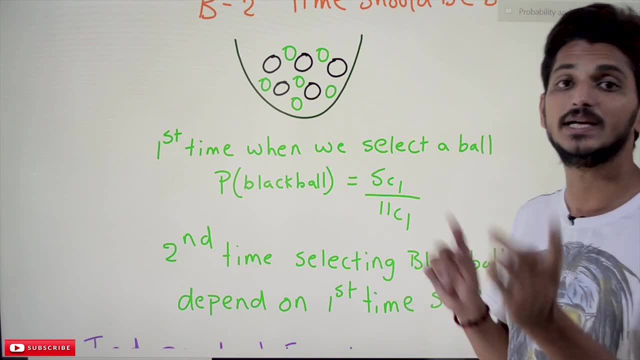 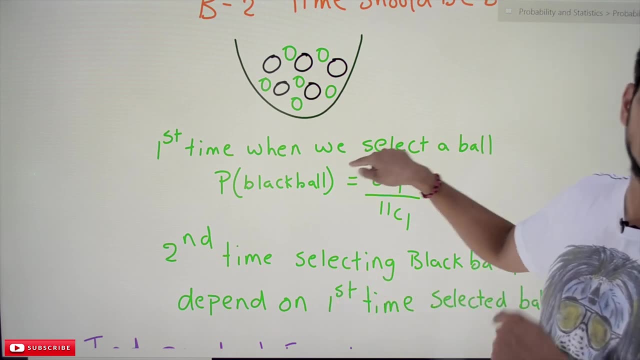 balls remain in the bag. Four black balls, Four c, one by ten c one is our next output. Second time, It completely depends on our first event, What happened in the first event. That is what dependent probability means, dependent events means. So how we find this dependency, how we find the 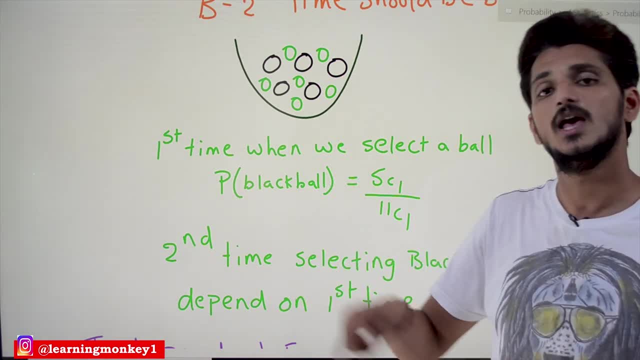 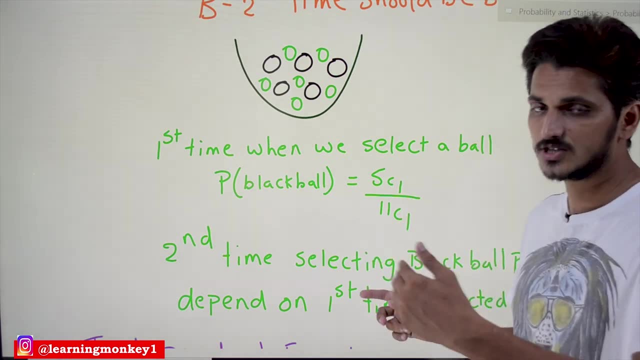 probability for dependent events will be discussed in our next class. when we discussed about conditional probability, We will go with conditional probability in this case. We are going to discuss about conditional probability in our next class. See here. what we are doing here is: 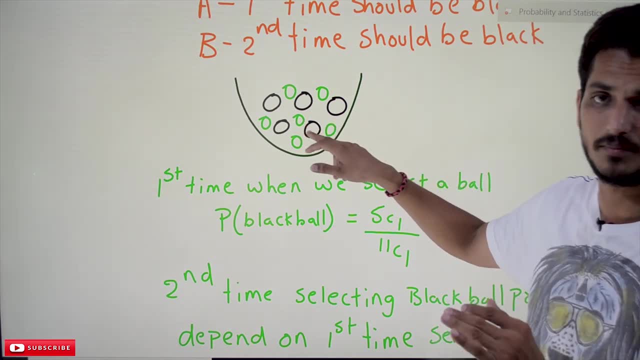 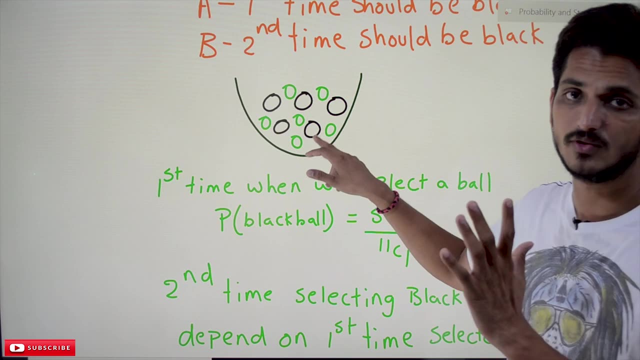 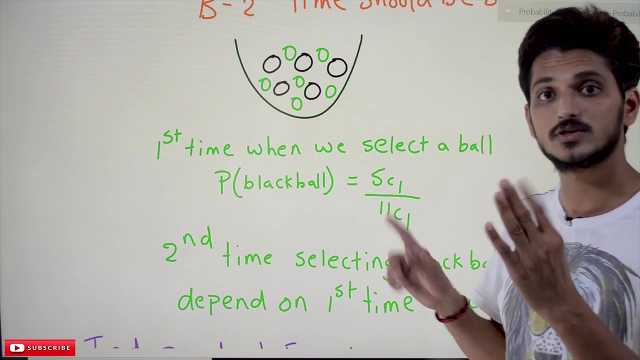 different, Because if you pick a green ball from this, how many balls remain? Total, ten balls will be there. How many black balls will be there? Five black balls will be there First time. if you select black ball, how many black balls remain in the bag? Four black balls, Four c one by ten c one is our. 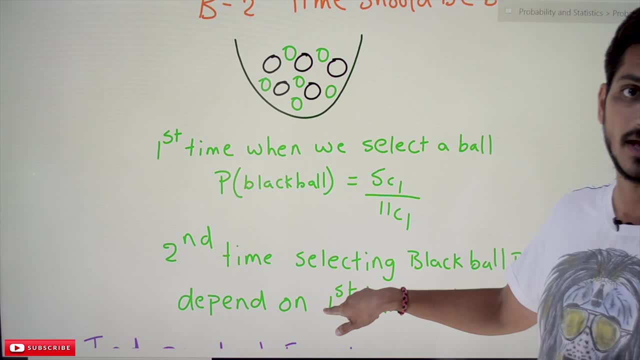 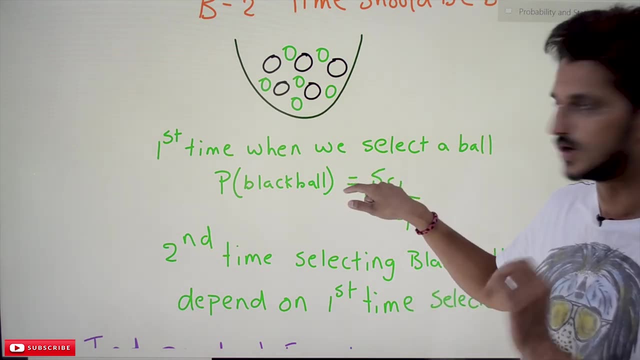 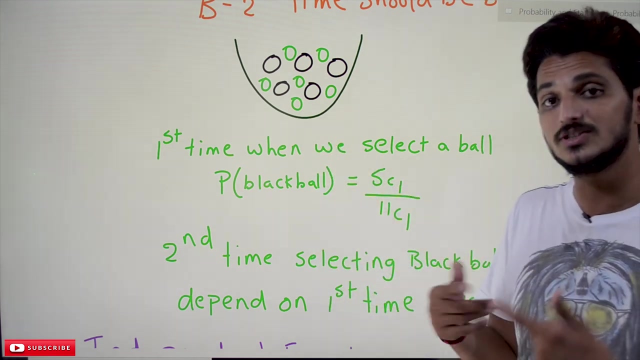 next output. Second time, It completely depends on our first event. What happened in the first event? That is what dependent probability is. Okay. Dependent probability means dependent events means. So how we find this dependency, how we find the probability for dependent events, will be discussed in our next class, when we discussed about 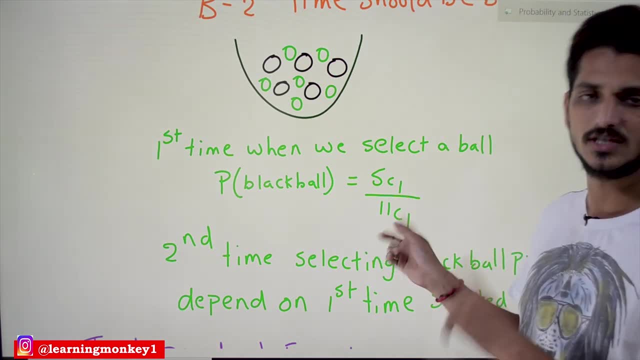 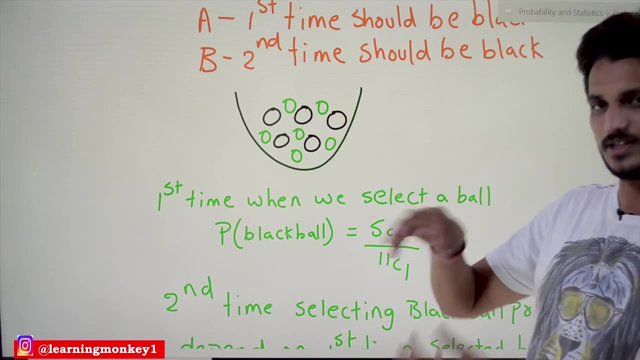 conditional probability. We will go with conditional probability in this case. We are going to discuss about conditional probability in our next class. See here: what we are doing here is first time. when you pick a black ball, you pick any ball. So first time, if you pick a ball, we are not going. 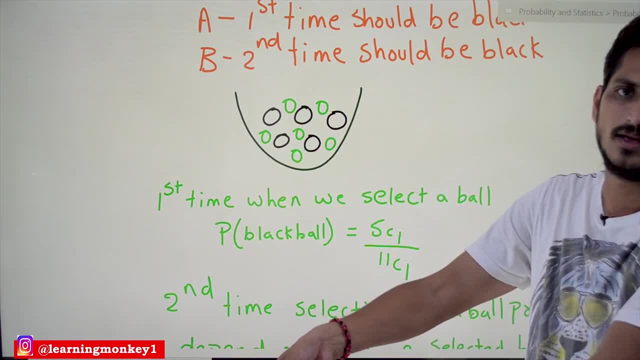 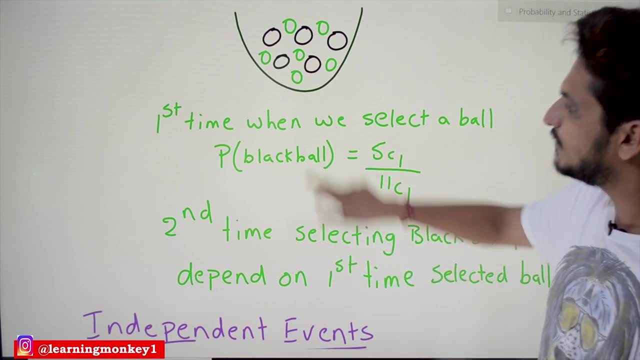 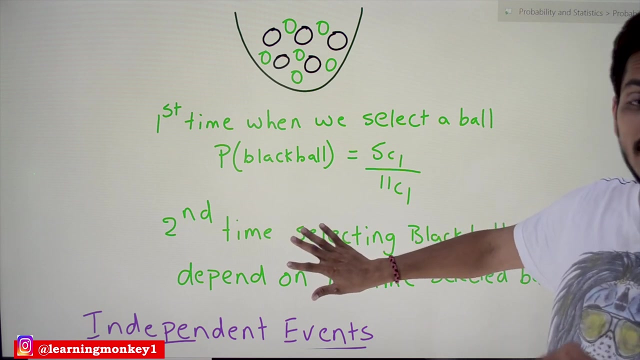 to replace the ball again in the bag. That is what this experiment says. If you replace the ball again back, then these two events are independent events, Because whatever happened here, the probability of picking a black ball second time is not changing because of this event, because we are replacing the. 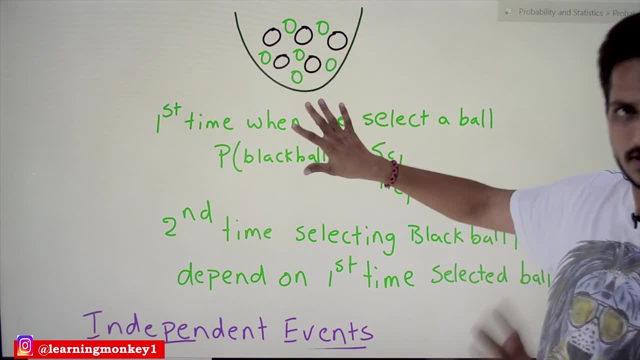 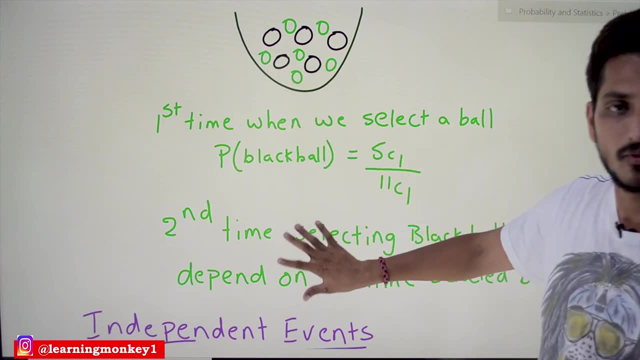 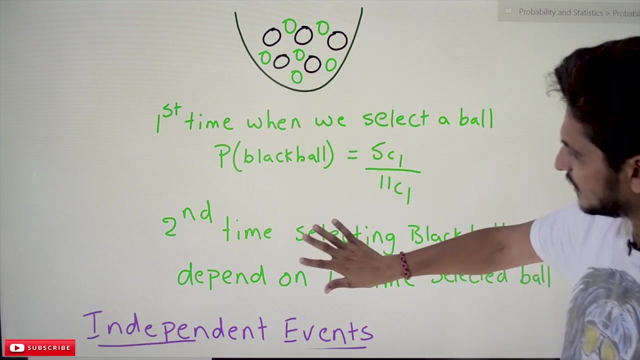 ball again First time. first time, what's the probability to pick a black ball- Five c, one divided by eleven c. one Second time if you replace the ball again? whatever ball you pick here, it doesn't matter. If you replace the ball again, what's the probability that second time you are going to pick a black ball? 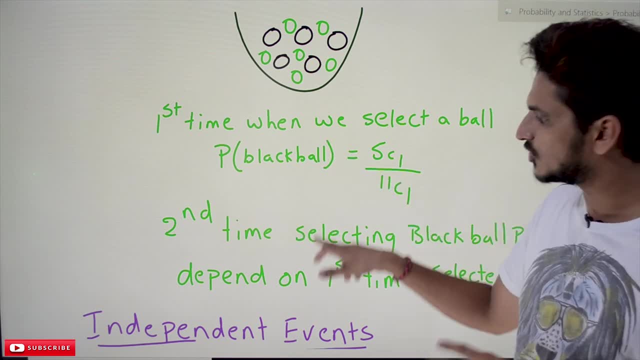 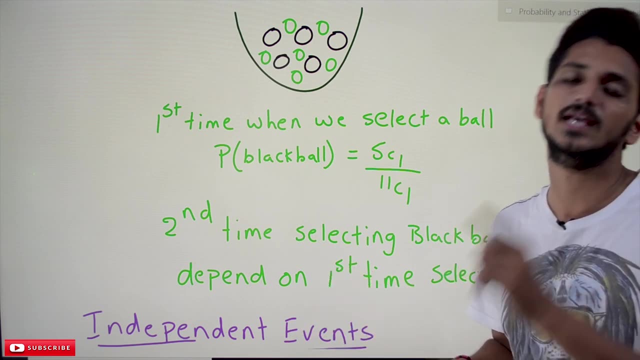 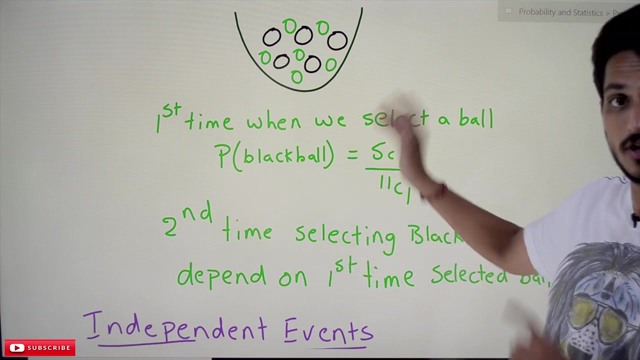 5C1 by 11C1.. This event is not going to affect the second event's probability. Then we say it as independent events. If you don't replace the ball, it is going to affect the second one's probability. If you replace the ball, it is not going to affect the second one's probability. 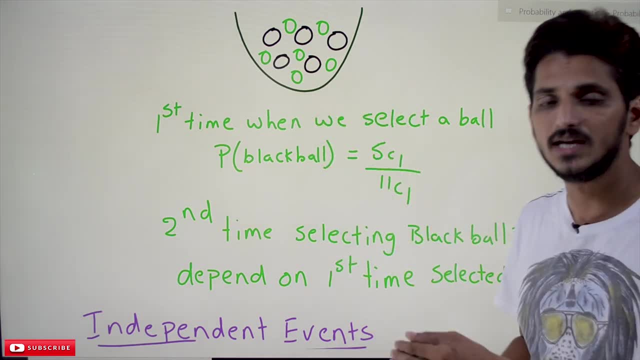 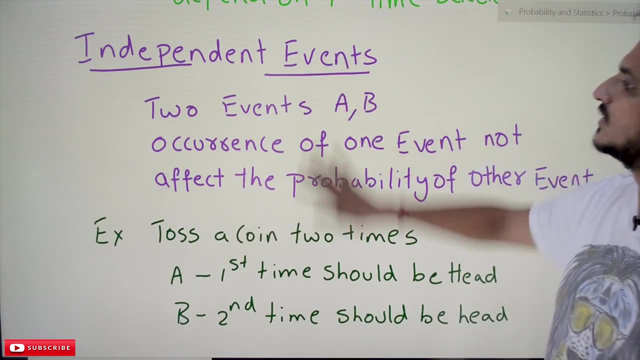 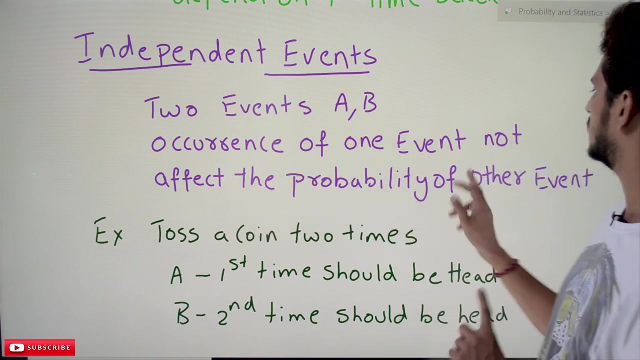 If you don't replace the ball, it is dependent events. If you replace the ball, it is independent events. Again, we are going to understand independent events with one more example. Two events, A, B, are said to be independent events. Occurrence of one event not affect the probability of other event. 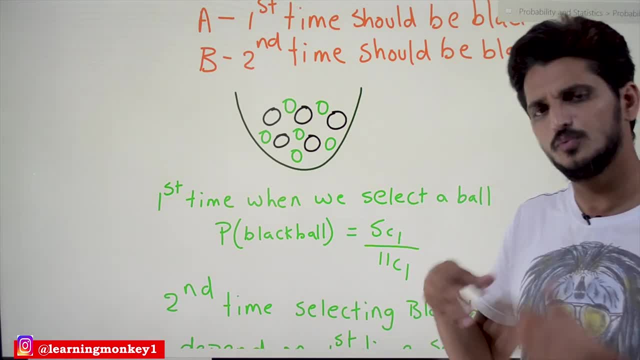 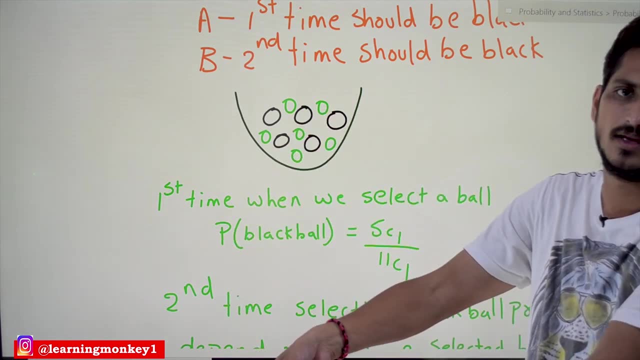 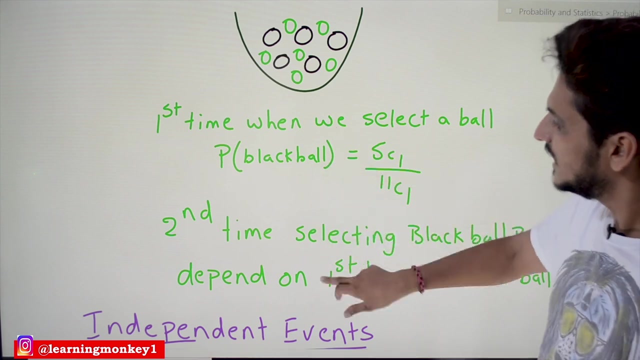 first time when you pick a black ball, you pick any ball. So first time, if you, if you pick a ball, we are not going to replace the ball again in the bag. that is what this experiment says. if you replace the ball again back, then these two events are independent events because whatever happened here, the probability of 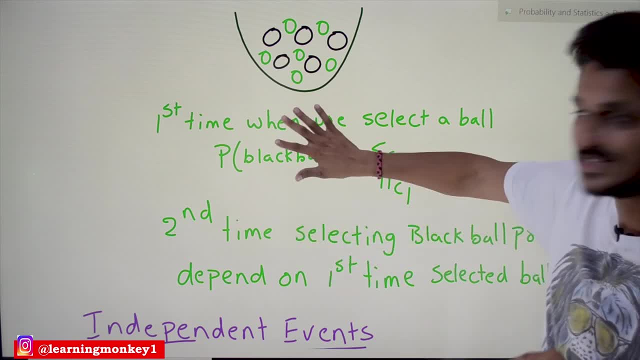 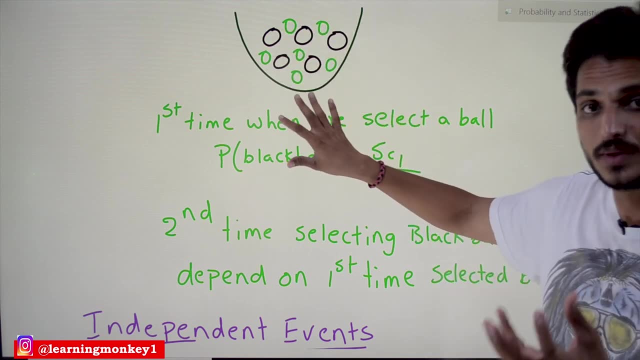 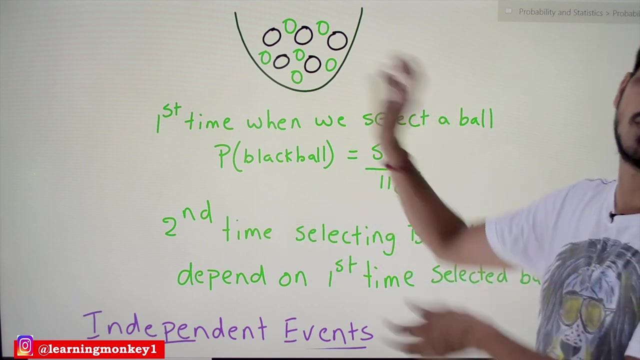 picking a black ball second time is not changing because of this event, because we are replacing the ball again first time. first time, what's the probability to pick a black ball- 5 c 1 divided by 11 c 1 second time? what if you replace the ball again? whatever ball you pick here, it doesn't. 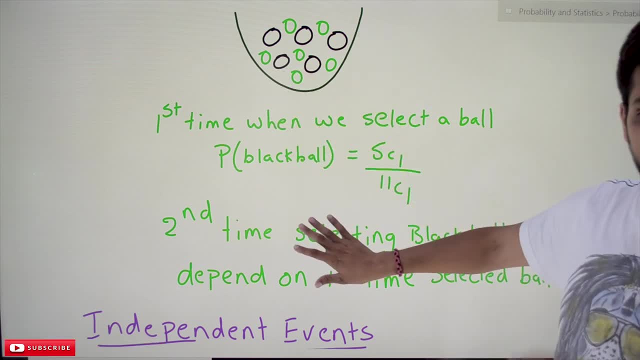 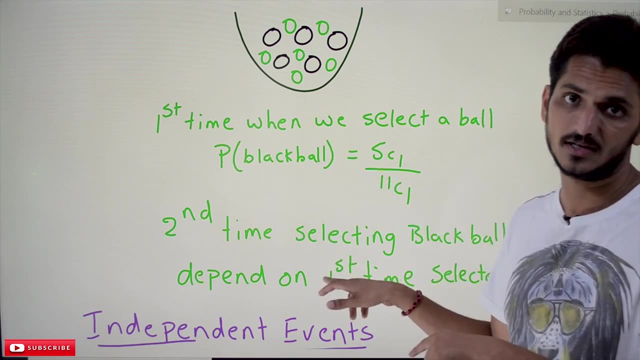 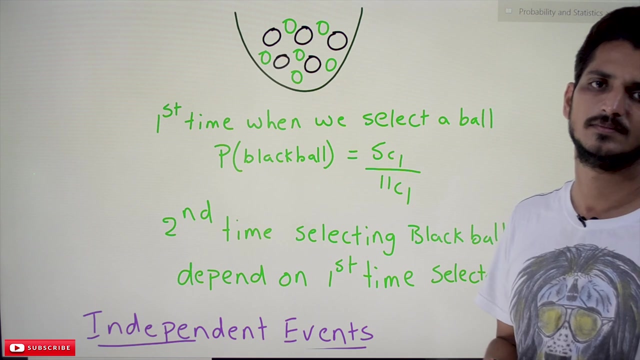 matter. if you replace the ball again, what's the probability that second time you are going to pick a black ball 5 c 1 by 11 c 1? this event is not going to affect the second events probability, then we say it as independent events. if you don't replace the ball, it is going to affect. 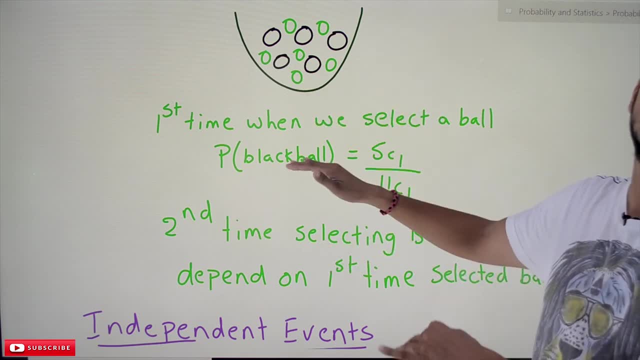 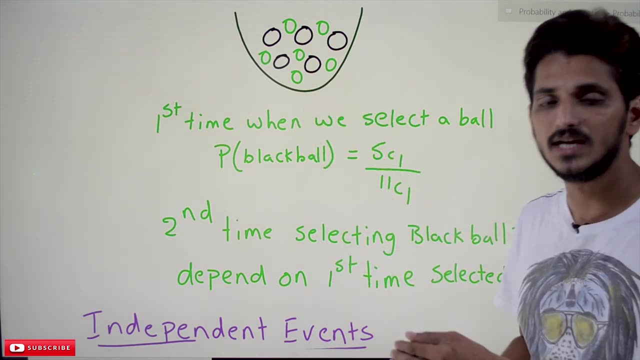 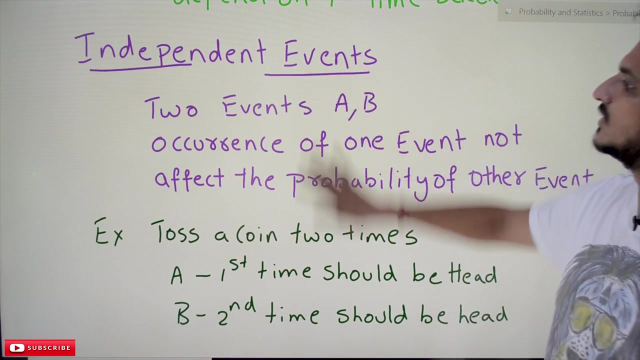 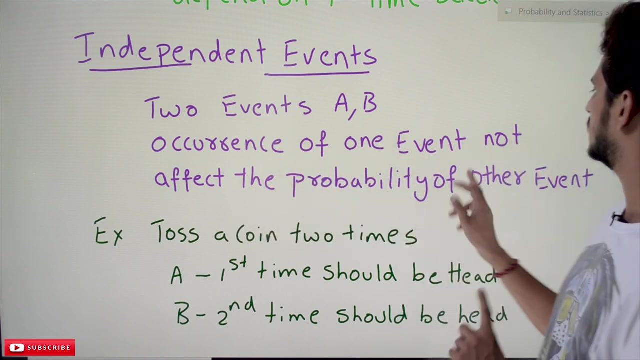 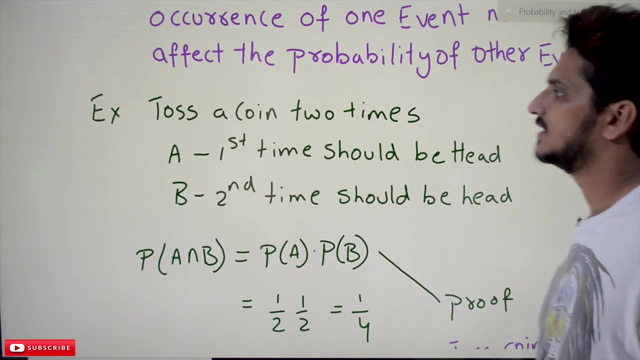 the second one's probability. if you replace the second one's probability, you will get a black ball: 5 c 1 divided by 11 c- 1. replace the ball. it is not going to affect the second one's probability. If you don't replace the ball, it is dependent events. If you replace the ball, it is independent events. Again, we are going to understand independent events with one more example. Two events, A B, are said to be independent events. Occurrence of one event not affect the probability of other event. Then we say it as independent events. Best example to understand independent events is: 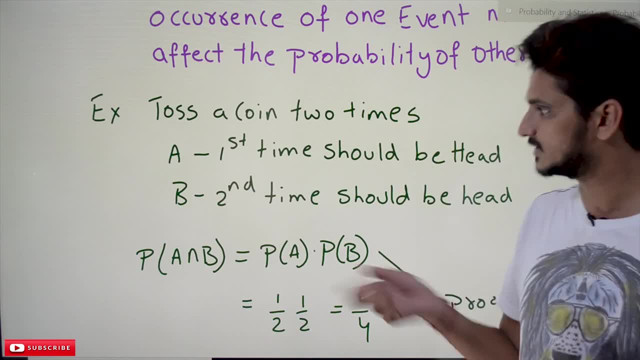 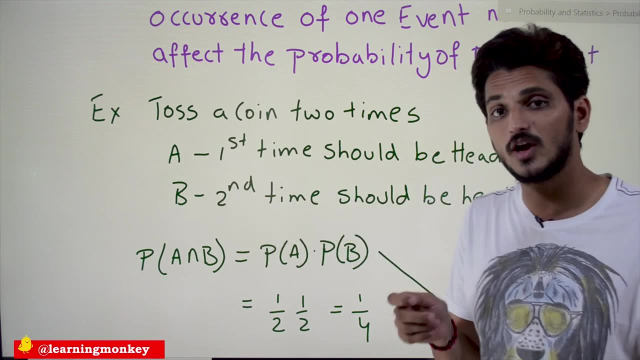 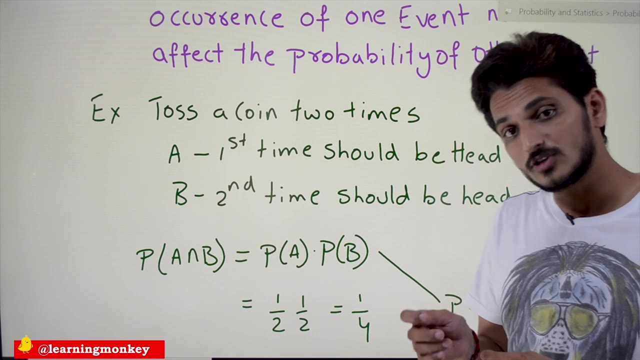 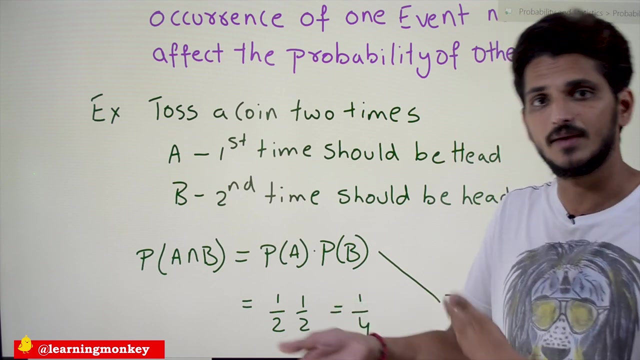 toss a coin two times. When you toss a coin first time, what's the event? A B event says that first time should be a head B, second time should be a head. When we toss a coin first time, what is the probability that it is going to be head 1 by 2.. When you toss the coin second time, what is the probability it is going to be head 1 by 2.. It is not going to affect the probability of head second time because the first event is not dependent on the second event. 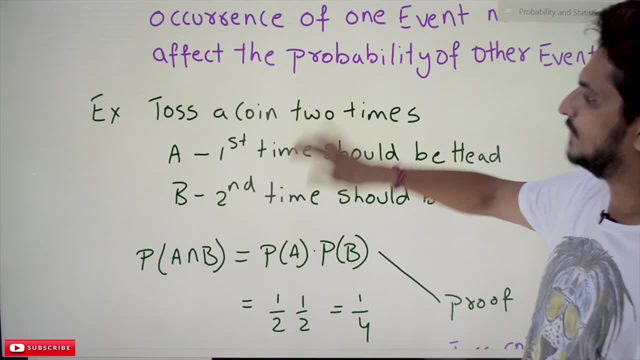 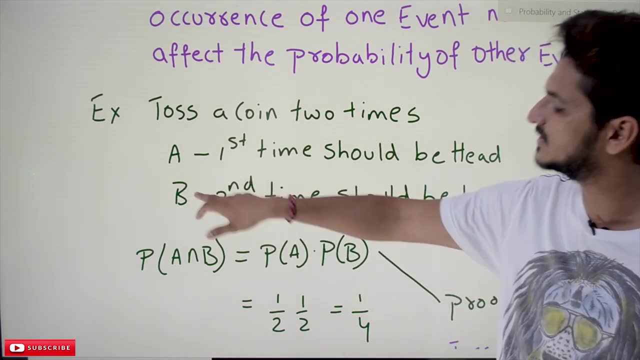 Then we say it as independent events. Best example to understand independent events: Toss a coin two times. When you toss a coin first time, what's the event? A B event says that first time should be a head B, second time should be a head. 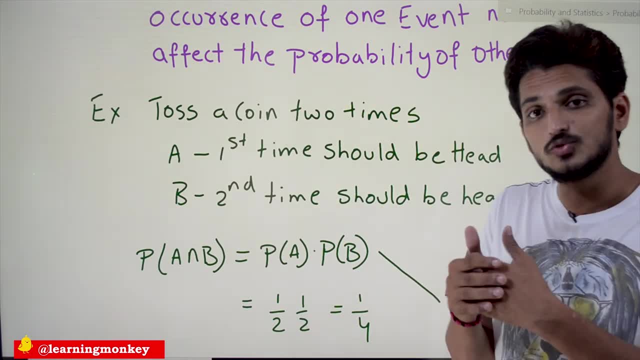 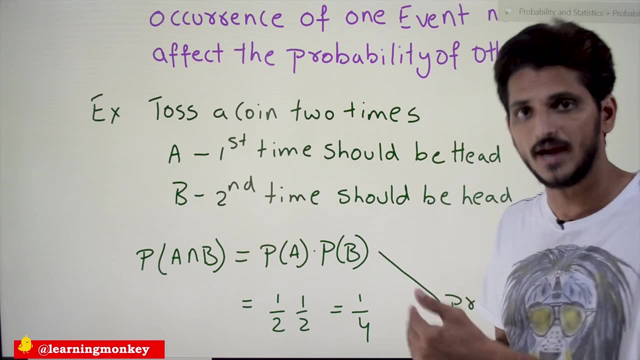 When we toss a coin first time, what is the probability that it is going to be head 1 by 2.. When you toss the coin second time, what is the probability? it is going to be head 1 by 2.. 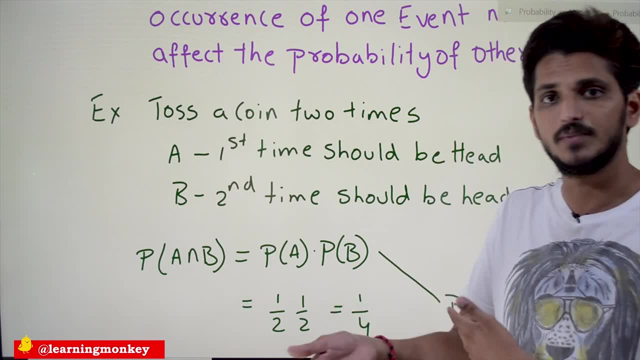 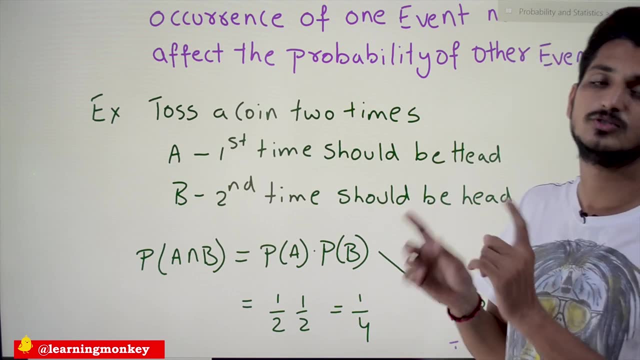 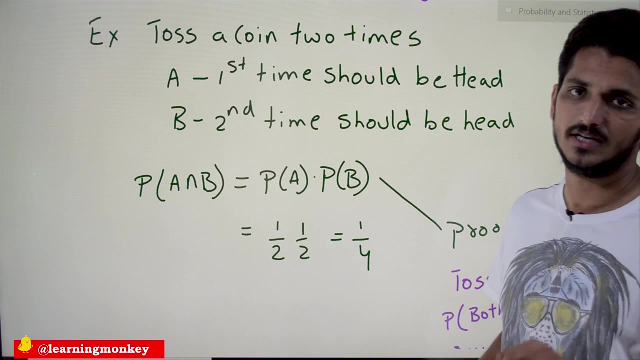 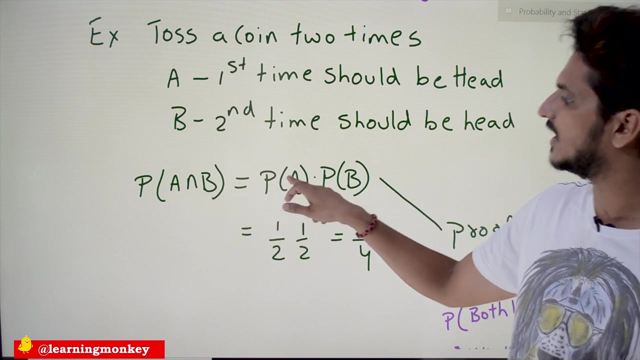 It is not going to affect the probability of head second time Because the second event is not dependent on the first event. That's why there are two independent events. If you are having independent events, how do we find the probability? Probability of A and B occurring of both the events is given as. 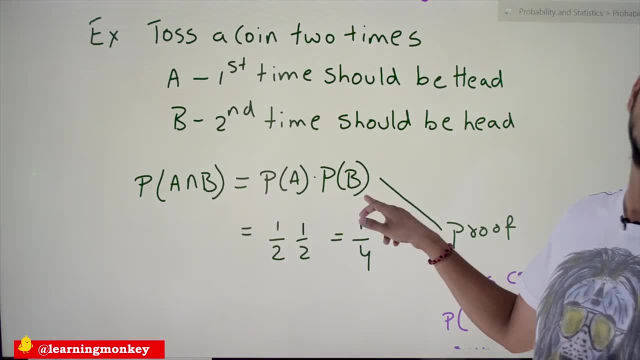 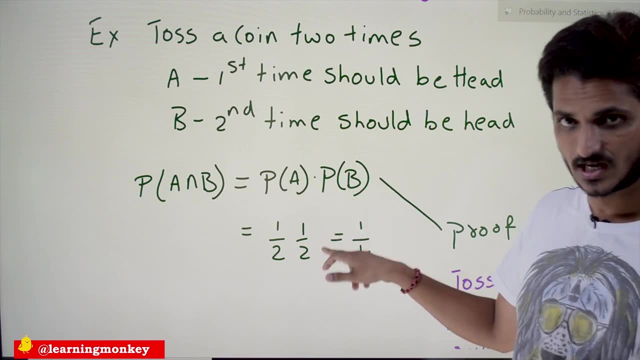 Probability of A multiplied by probability of B. What is probability of A Occurring of head for the first time is 1 by 2.. What is probability of B Occurring of head for the second time is 1 by 2.. 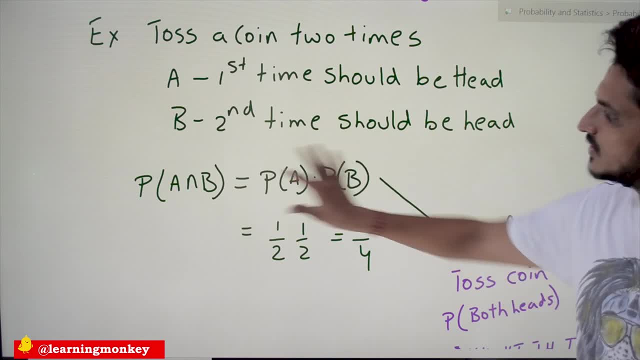 1 by 2 multiplied by 1 by 2 is 1 by 4.. This is the equation for if you are having independent events, probability of A and B- both events to occur- is equal to probability of A multiplied by probability of B. 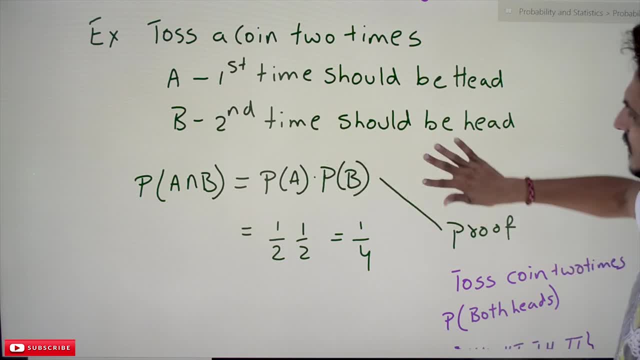 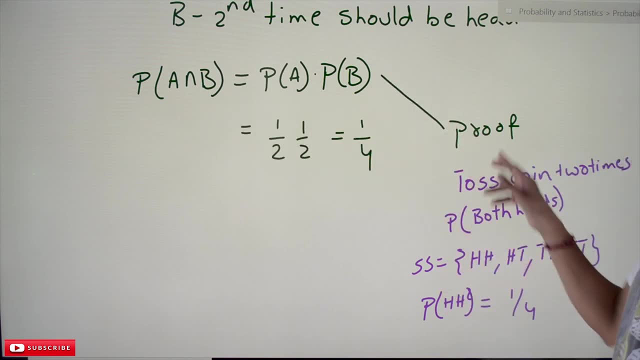 So we will go the proof of this with an example. So this is the independent events formula. Without this formula, if you try to do the example, toss coin two times probability of both heads. So if you toss coin two times, what is our sample space? 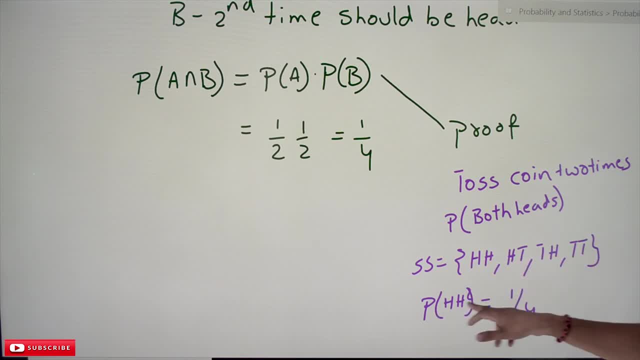 Head head Head tail, Tail, head, Tail, tail, Tail, tail. Probability of head head is out of these four chances, head head is having one chance, So 1 by 4.. Here we got the same output. 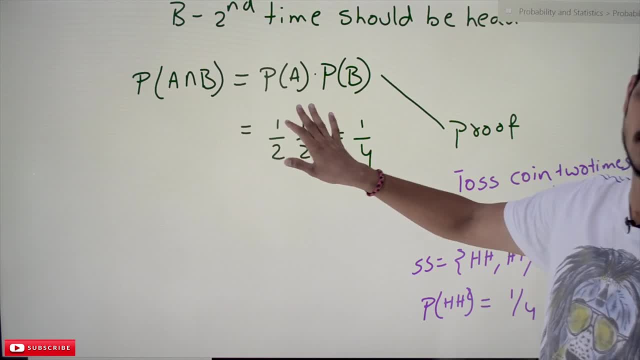 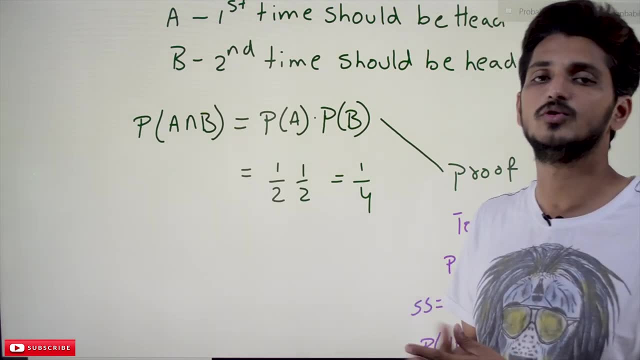 So that is why this is what the equation for independent events. For dependent events, the equation is different. We are going to discuss about conditional probability in our next class. After that we are going to do many examples based on this conditional probability and 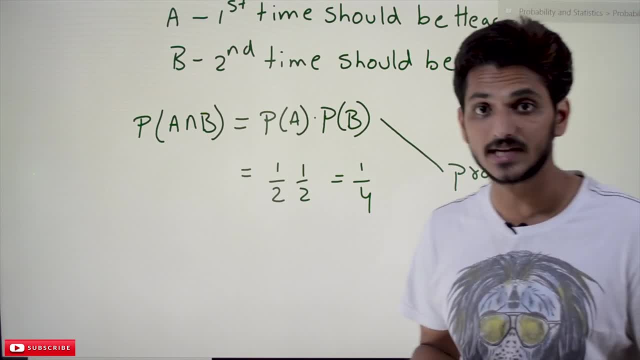 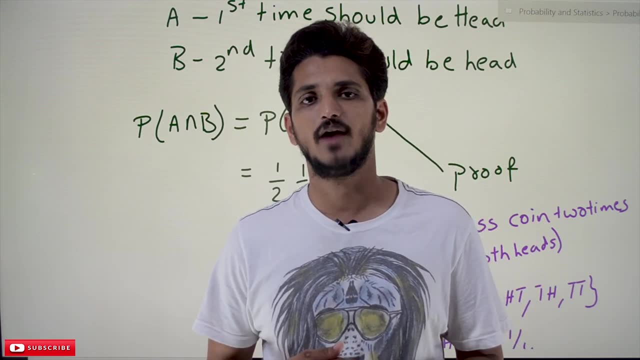 remaining examples also Hope you understand the concept of dependent and independent events. If you have any questions regarding the concept, please post your questions in the comment section below. Thanks for watching. If you haven't subscribed to our channel, please subscribe to our channel and press. bell icon for the latest updates. Thank you.